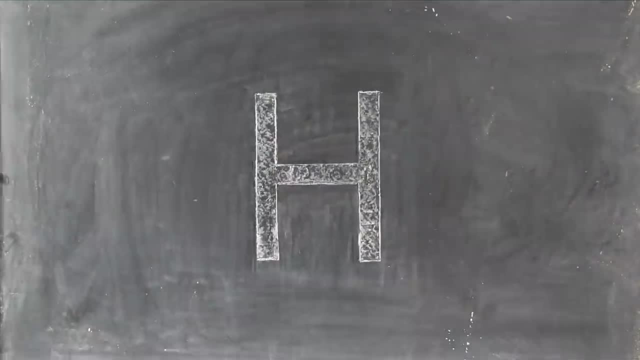 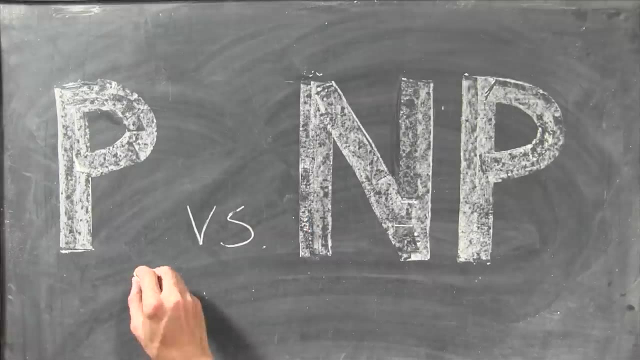 Today I want to talk about the deepest unanswered question in computer science and maybe in all of math, a problem called P versus NP. And I want to talk about how ideas from computing show up in the everyday world around us and how problems as seemingly disparate as protein 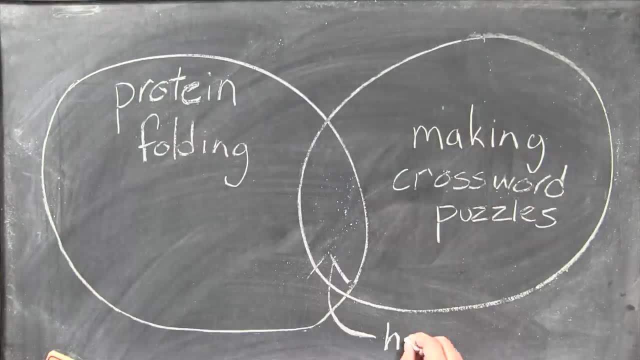 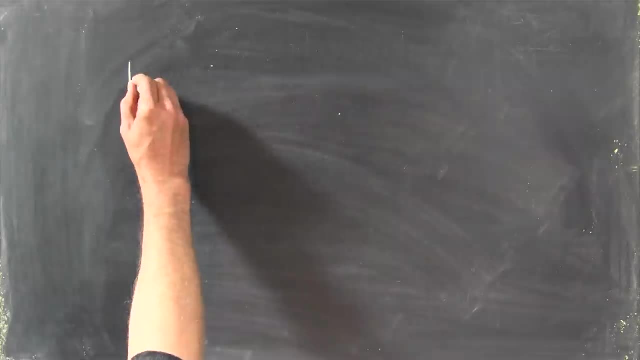 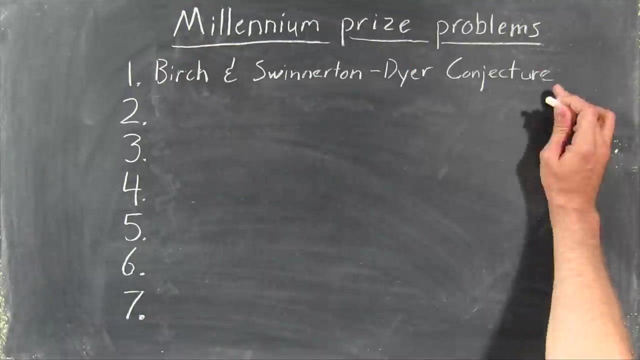 folding and making up crossword puzzles share a common core difficulty. that turns out to be a lot like Sudoku. Well, basically it is Sudoku. In 2000,, the Clay Institute offered $1 million each for the solutions to seven key problems in math, the Millennium Prize problems. These are profound and difficult problems and for 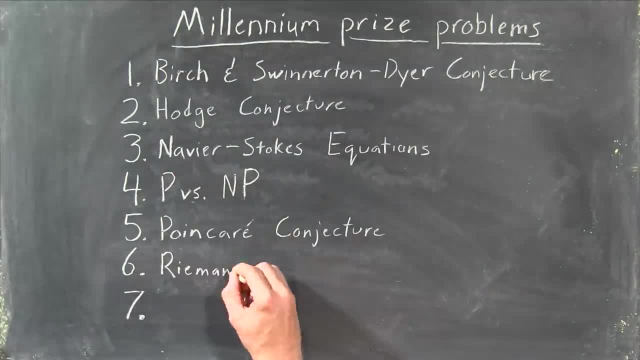 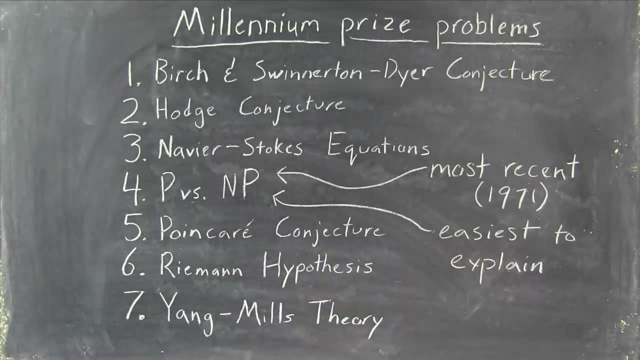 most of them, it takes a lot of specialized knowledge to even understand. the question Of the seven problems P versus NP was both the most recently conceived, in 1971, and by far the easiest one to understand and explain, And in March 2010,, the Clay Institute awarded 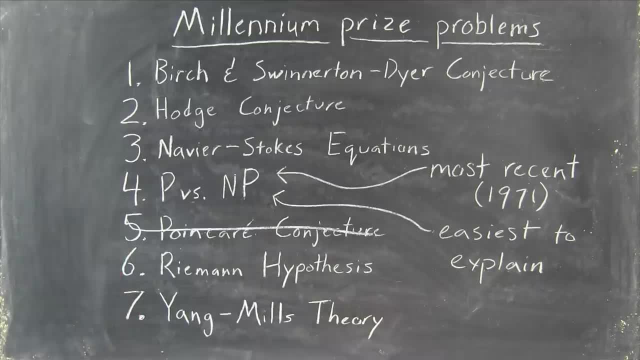 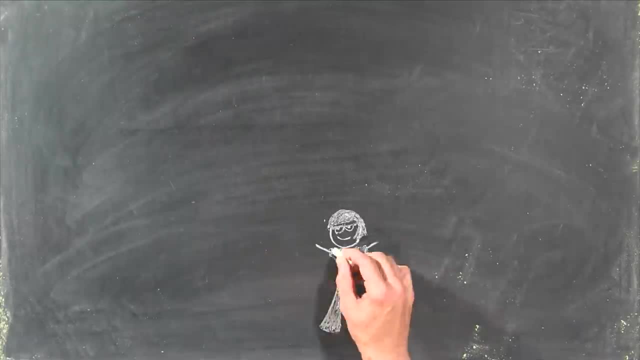 the first of its seven prizes for the solution to yeah, not P versus NP. So what is the P versus NP question? Well, back in the 70s, computer scientists were busily figuring out how to solve the problem, And in the 1970s they were able to solve. 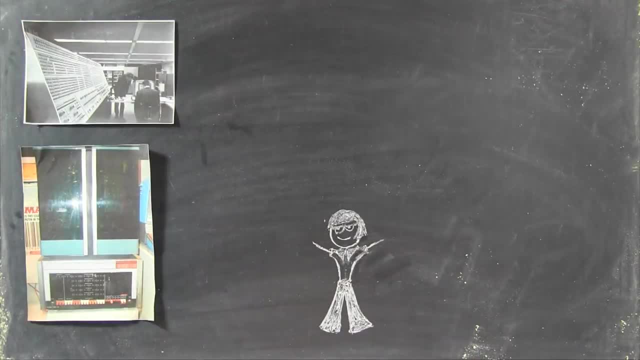 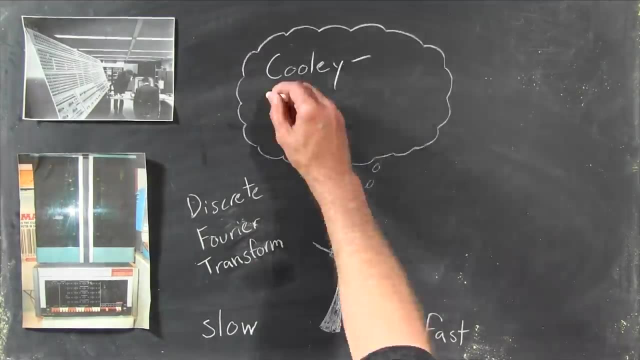 out how to program their retro-fabulous cabinet-sized computers to solve all the world's problems. Sometimes the first program anyone could think of for a particular problem would be unworkably slow, but then over time people would come up with clever ways to make it faster. Or 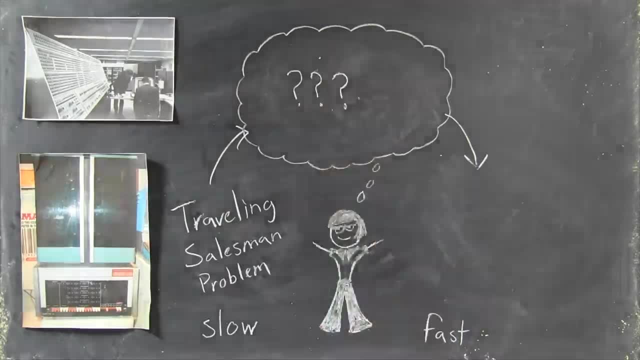 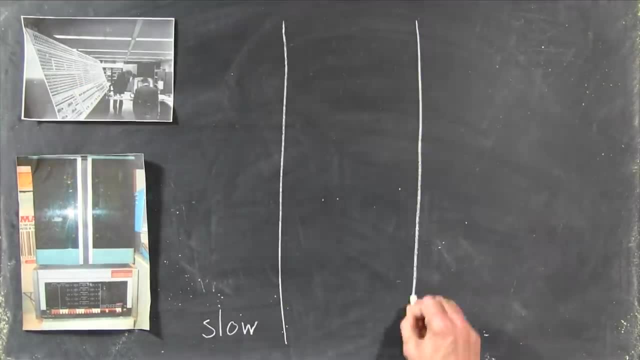 at least that happened for some problems. For others nobody was coming up with faster programs. To get a handle on the situation, they started sorting the problems into classes based on how fast a program could solve them. For problems like multiplication they had. 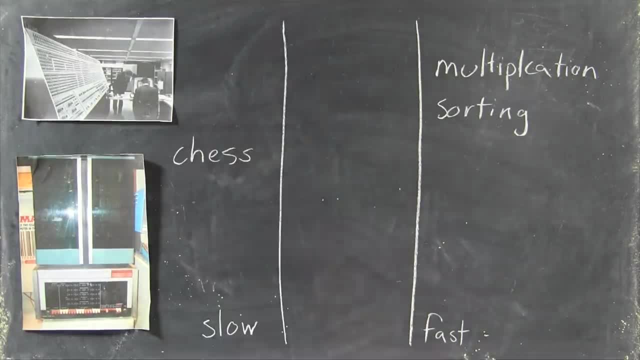 really fast programs and for others, like playing absolutely perfect chess, they had to figure out that there just was no fast program. But for a bunch in between they weren't sure whether there was a fast way to do it, So they kept trying. 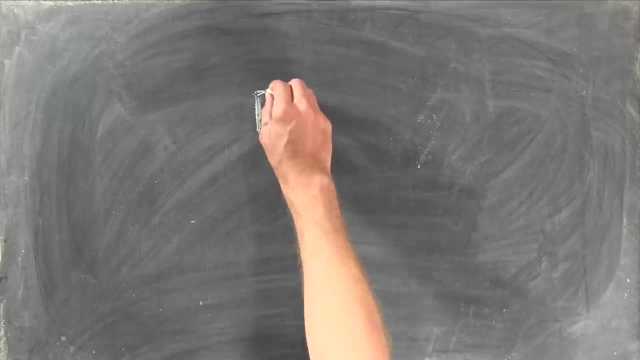 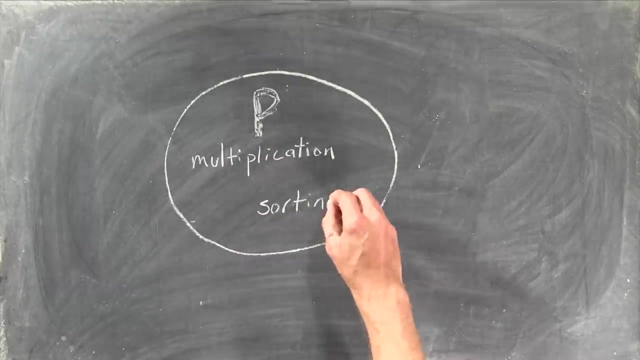 This is where P and NP come in, Skipping a ton of details for a second. P is a class that basically includes all the problems that can be solved by a reasonably fast program, like multiplication or alphabetizing a list of names And then around and including P. 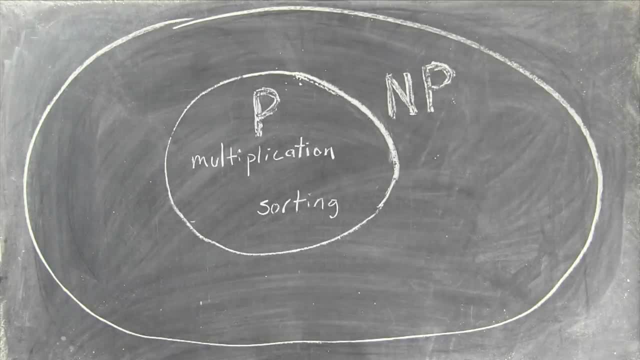 we sort of discovered a class called NP. That's all the problems where if you're given a correct solution, you can at least check it in a reasonable amount of time. NP was the totally maddening because it contained lots of important problems like vehicle routing. 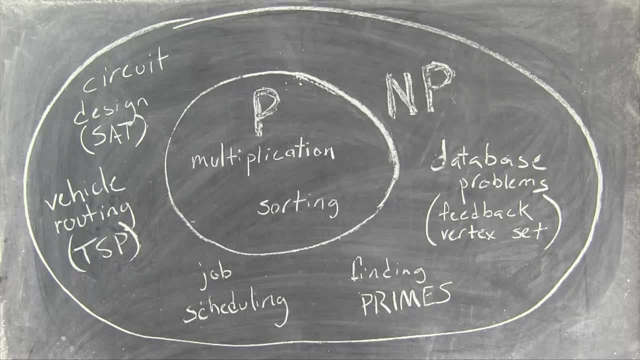 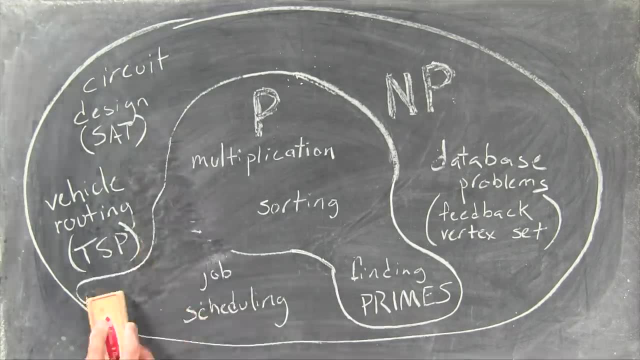 and scheduling and problems in circuit design and databases, And often we'd get lucky and find that an NP problem was actually a part of P and we'd have our fast program. But for a lot of them that didn't seem to be happening. So people started to wonder whether 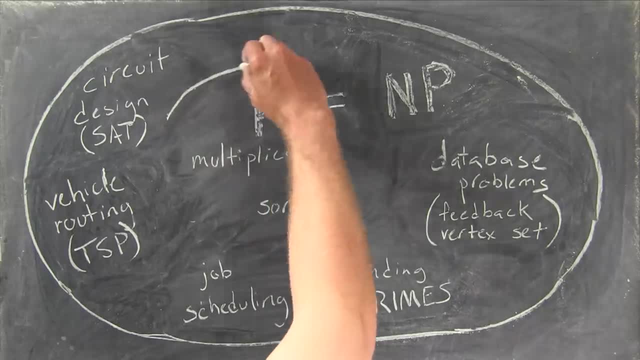 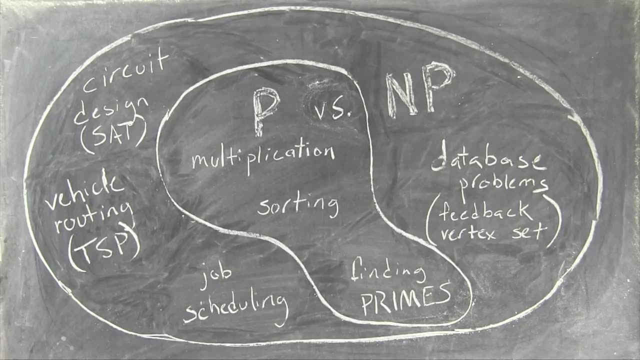 everything in NP would turn out to be in P, or if there were some NP problems that were truly harder than the ones in P. That's the P versus NP question, If all the NP problems are really in P. a lot of important puzzles we've been struggling. 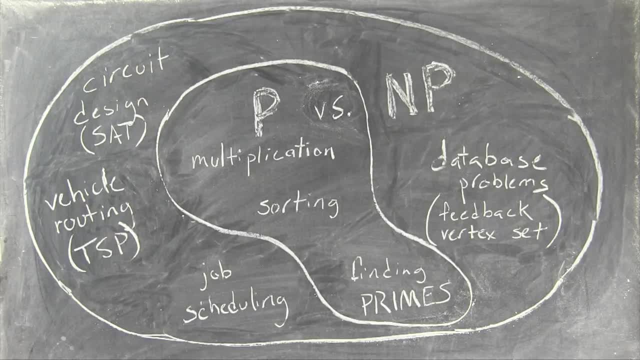 with are going to turn out to be easy for computers to solve. Puzzles connected to biology and curing cancer, puzzles in business and economics. we'd have a lot of miracle answers almost overnight, And also the encryption we use for things like online banking would. 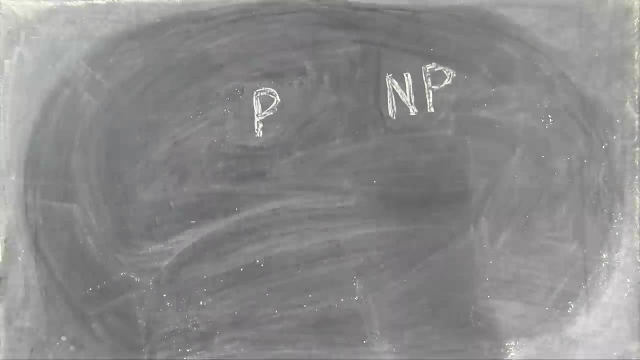 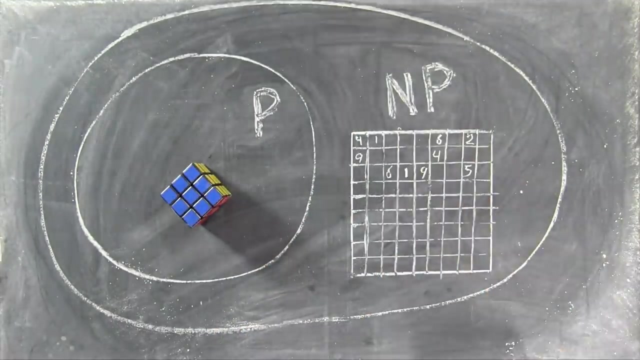 be easy to crack because it's based on NP problems. Okay, examples: I like to think of the problems in NP as being basically like puzzles, because I think what makes a puzzle a puzzle is that it's a problem where you can give away the 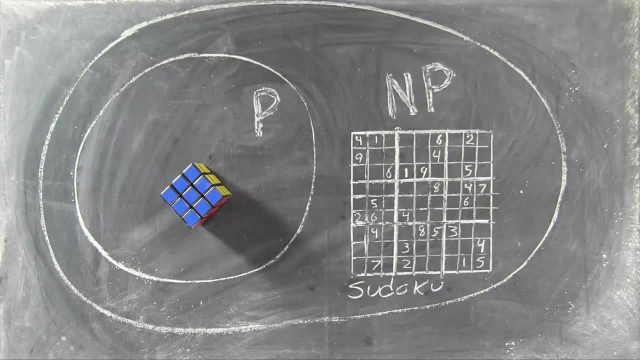 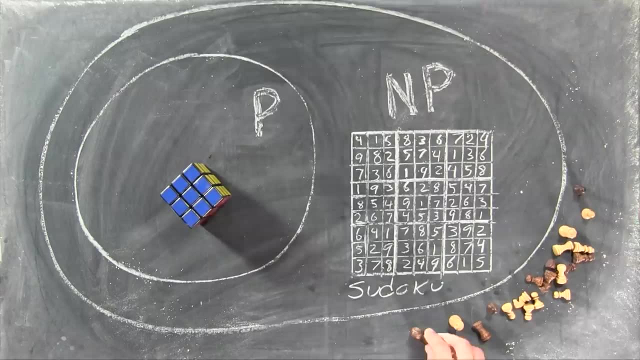 answer, And that's what NP means, Like with Sudoku. Sudoku puzzles can take a long time to solve, but if I give you a solved Sudoku grid, checking it for mistakes is pretty quick. Outside of NP are problems where it's hard to even check an answer, Like what's the? 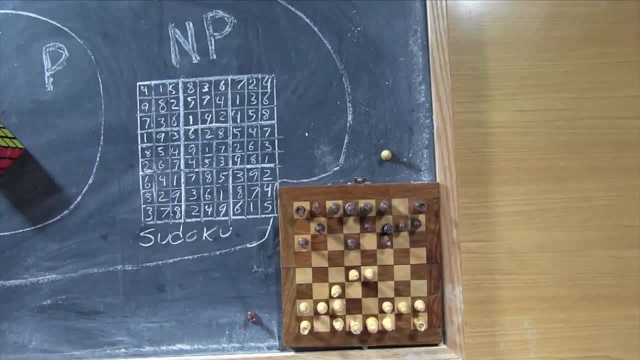 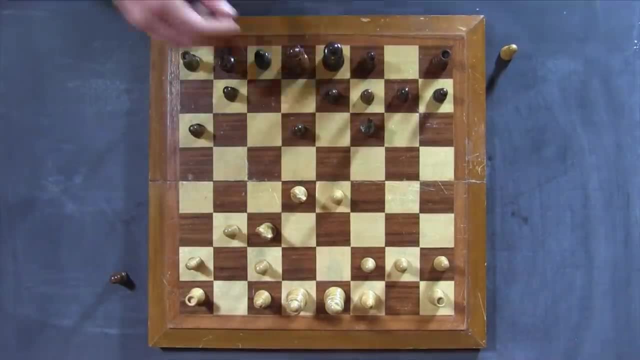 best move to make in this chess game. I could tell you the answer, but how would you know whether I'm right? Well, you wouldn't, because finding out requires a calculation so enormous that there's a pretty good argument: we'll never be able to build a computer that could. 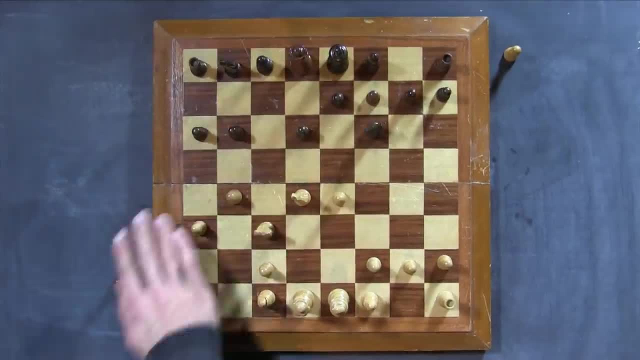 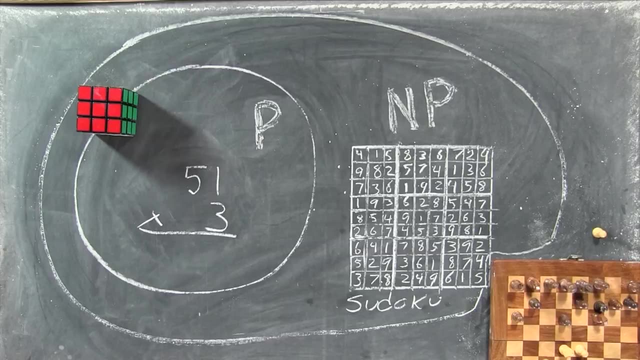 do it. To me that's not a very good puzzle. It's practically impossible to know whether you've solved it. On the other side are all the reasonable solvable puzzles in P. These are also in NP because one way to check an answer is to go through the process of 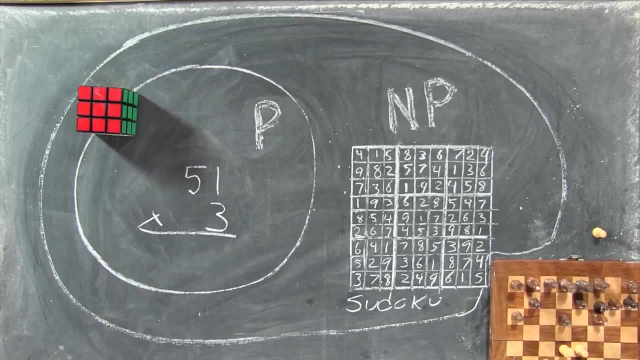 finding it yourself. Like if I were to tell you that the answer to 51 times 3 is 153,. how would you check whether I'm right? You'd probably just multiply 51 by 3 yourself, because it's fast to do it. But Sudoku is different, Or at least we think it is. It seems like solving. 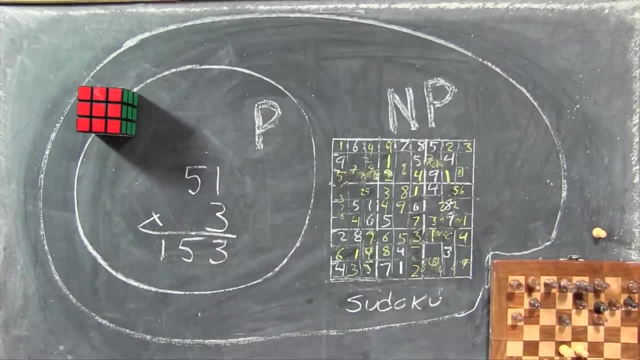 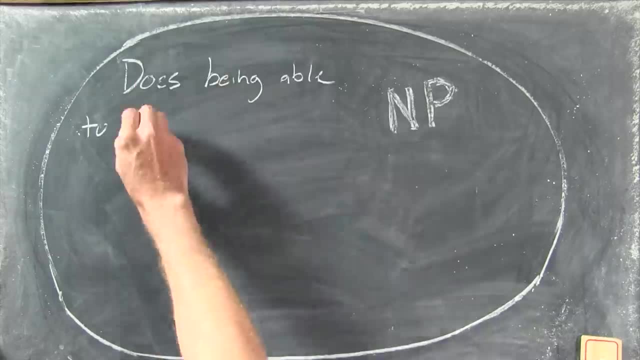 a Sudoku grid is a lot harder than checking a solution, but in fact nobody's been able to prove it yet. As far as we know, there could be a clever way of playing Sudoku much, much faster. Does being able to quickly recognize correct answers mean there's also a quick way to 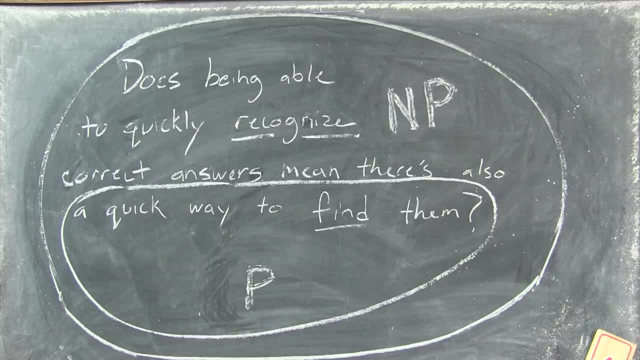 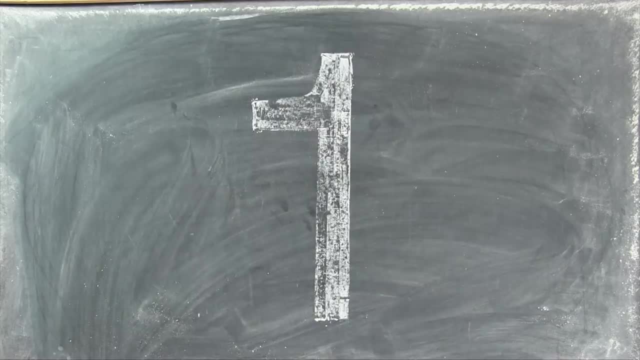 find them. Nobody knows for sure, but either way, figuring out exactly how this works would teach us something important about the nature of computation. It gets weirder from here. but first three important details. One: you might be thinking: hey, Sudoku is tough and all, but it's not that hard. What's? 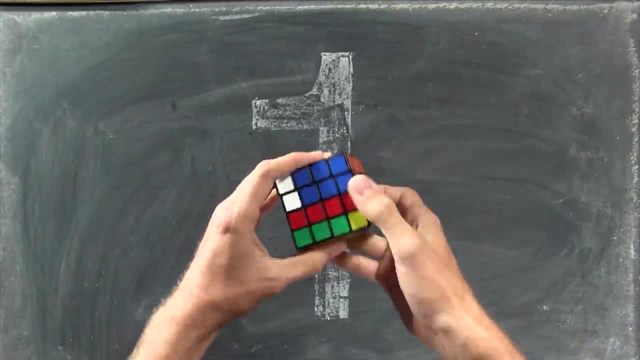 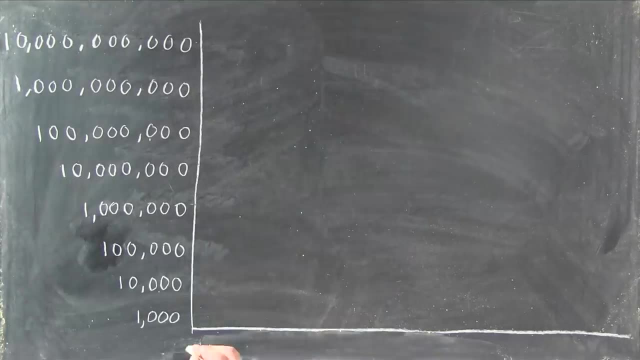 the big deal. Well, we're really talking about how the difficulty scales up as you make the problem bigger and bigger, Like how much harder is a 100x100 Sudoku grid than a standard 9x9 grid? We've been making computers exponentially faster as time goes on, so for problems that 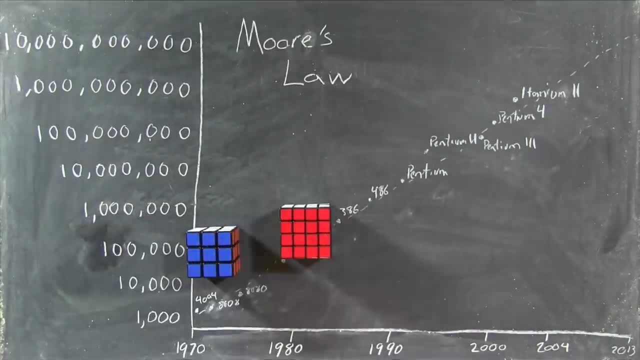 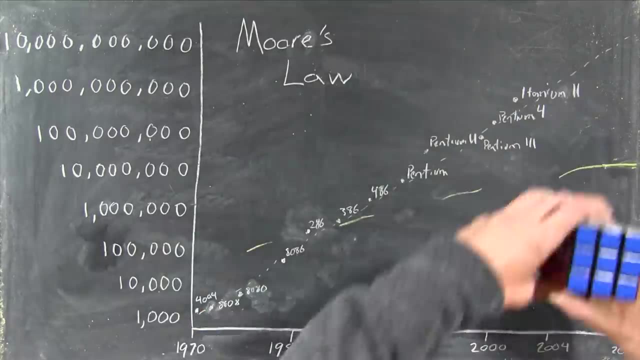 don't get exponentially harder as they get bigger. all we have to do is wait for computers to get more powerful and then even huge versions of those problems will be easy to solve by computer. Like multiplication problems are pretty easy for computers, even with enormous. 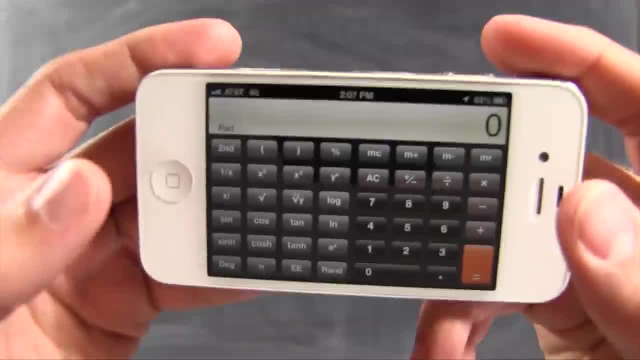 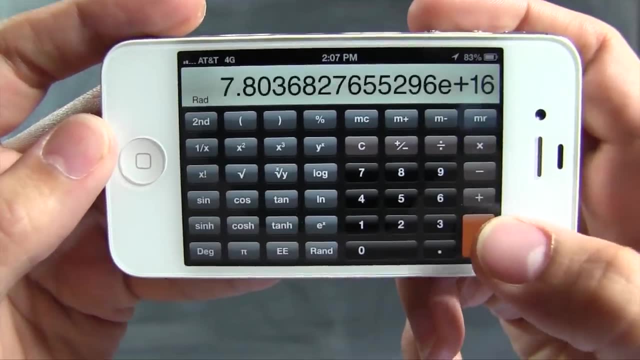 numbers. As the numbers get bigger, multiplying them just doesn't get harder very fast. These days, the phone in your pocket is what would have been referred to in the 1970s as a supercomputer, and you'd have to make a truly huge multiplication problem to stand up to all the computational problems. 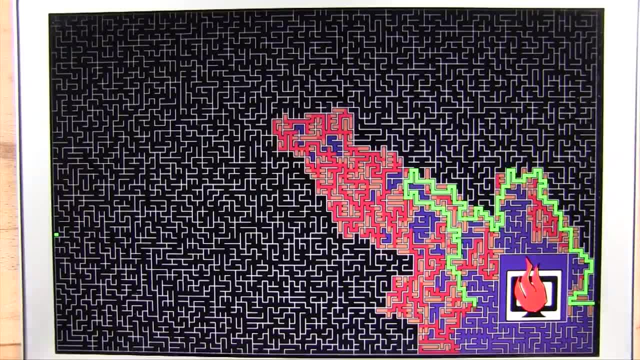 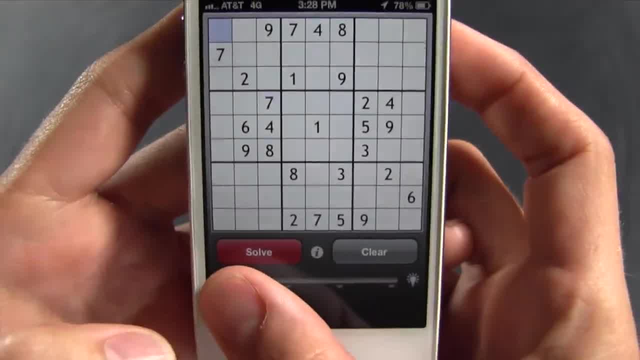 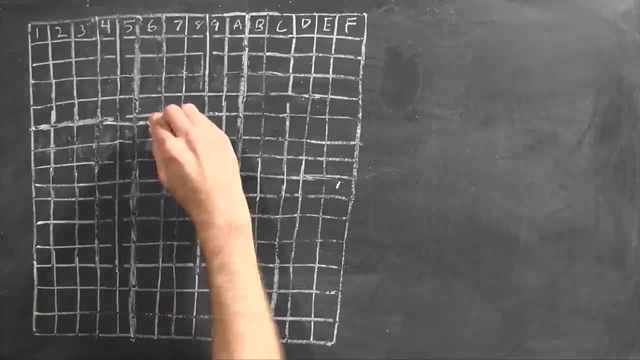 And then there's Sudoku. Computers can usually solve a normal 9x9 grid in a few milliseconds, even though humans find them challenging. But as you make the grid bigger, the problem just gets really hard, rapidly getting out of reach for even the most powerful computers. 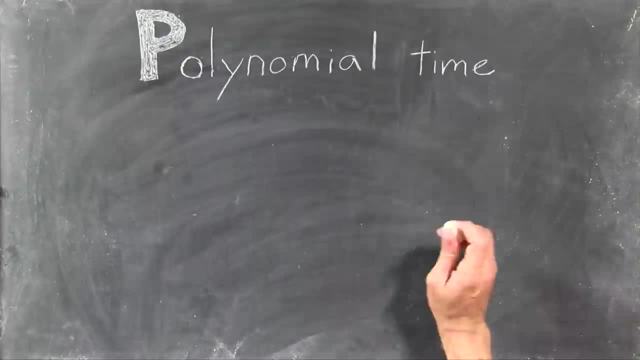 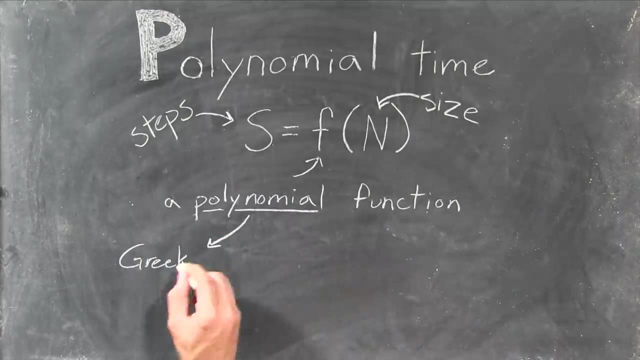 Two P stands for polynomial time. In P, the number of steps you have to do to solve a problem and therefore the amount of time that it takes, is some polynomial function of its size. Polynomial is a mishmash of Greek and Latin meaning many names, which is regrettably. 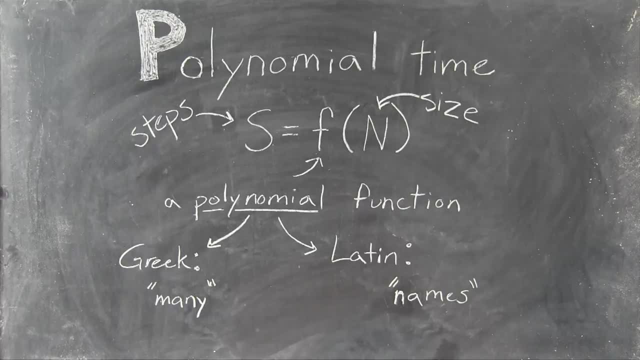 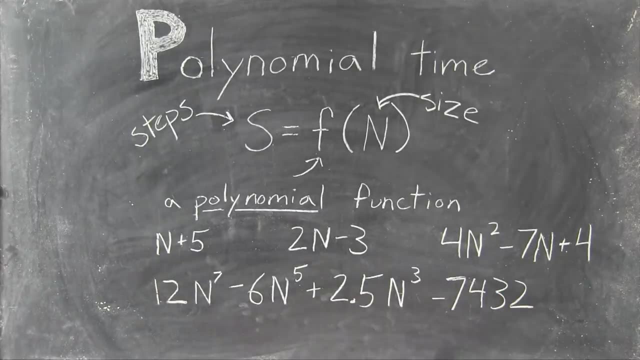 a pretty typical example of math's flair for unhelpful terminology. Anyway, polynomials are functions involving n or n squared, or n to other powers like these, But importantly they're not exponential functions like 2 to the power of n, which gets to be a ton. 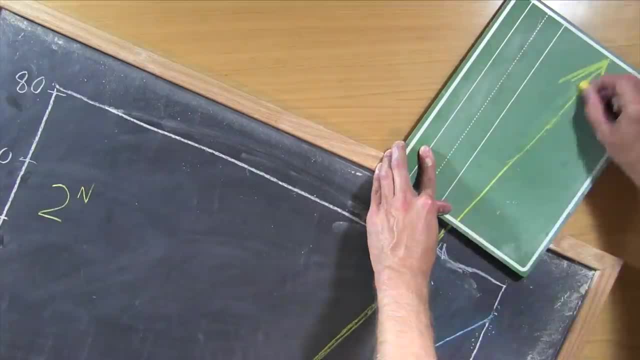 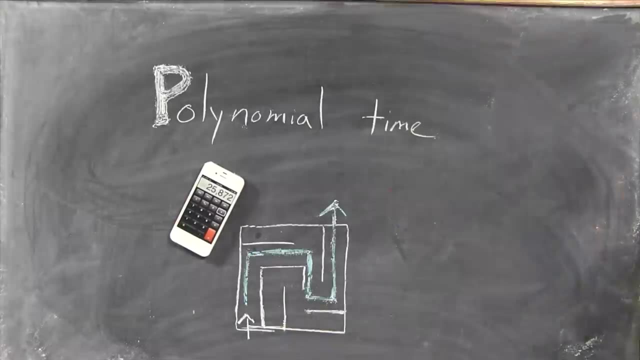 of steps really fast, as n goes up a lot quicker than n to the power of 2.. So that's P. It's problems like mazes and multiplication, where the number of steps required isn't that bad compared to the size of the problem. 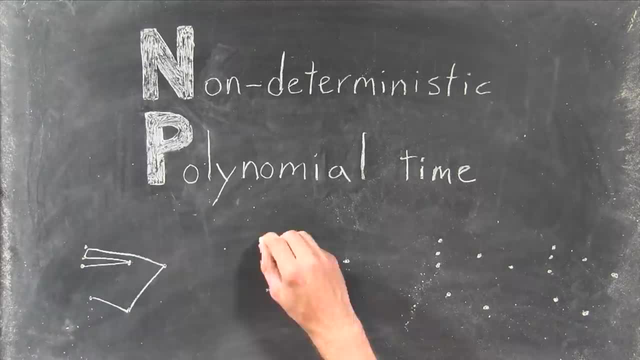 NP is all about polynomial time checking. NP stands for non-deterministic polynomial time, which, being math terminology, is an almost mean-spirited way of saying that if you had a bajillion computers and you could check all possible answers at the same time. 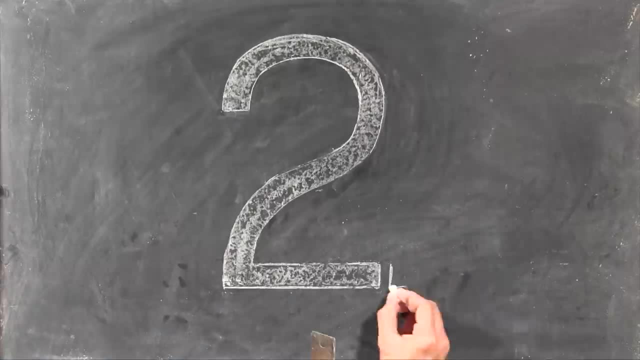 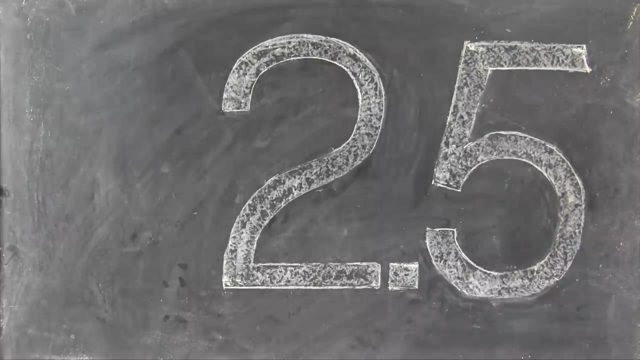 you could find a correct solution in polynomial time. Two point five. We're actually talking about the number of steps required to solve a problem in the worst-case scenario, Like how many steps does it take to unscramble a Rubik's? 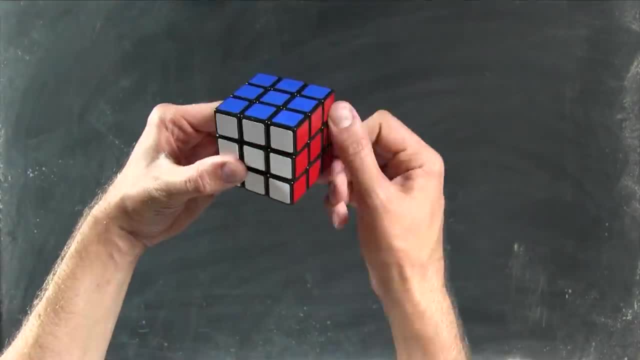 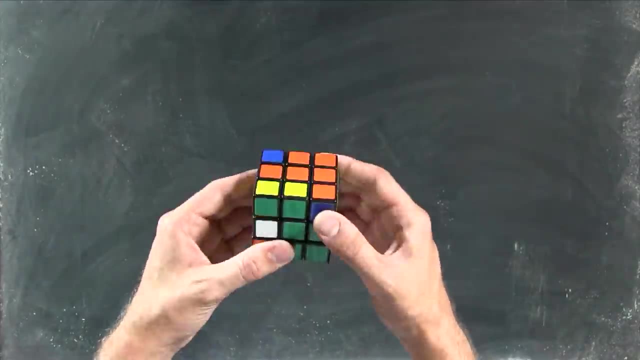 Cube. Well, when it's scrambled like this, it takes one step, But it can get a lot worse. Similarly, some 9x9 Sudokus are harder than others. People also look at things like the best case and the average case, but worst-case analysis. 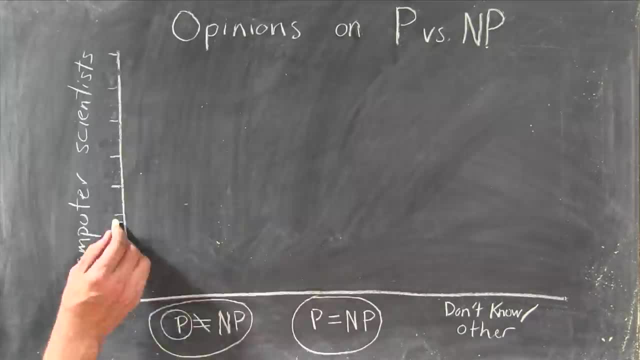 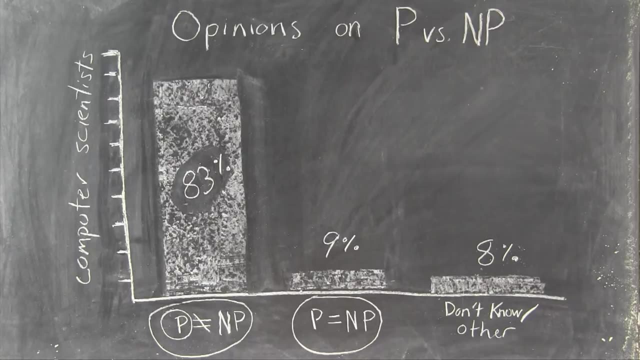 is what we know the most about Three. Actually, pretty much everybody thinks it's obvious that NP contains more problems than P. It's just that we haven't been able to prove it. The bad news for fast solutions came in the early seventies, when complexity researchers realized that dozens of those 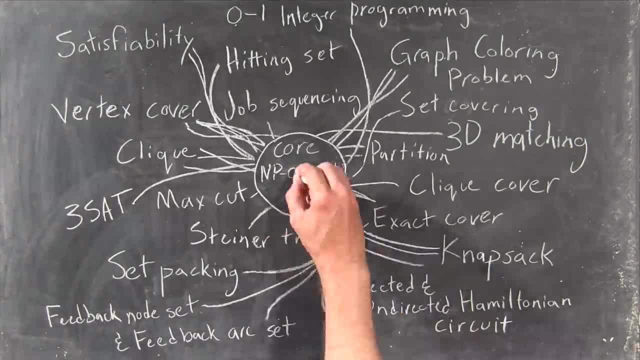 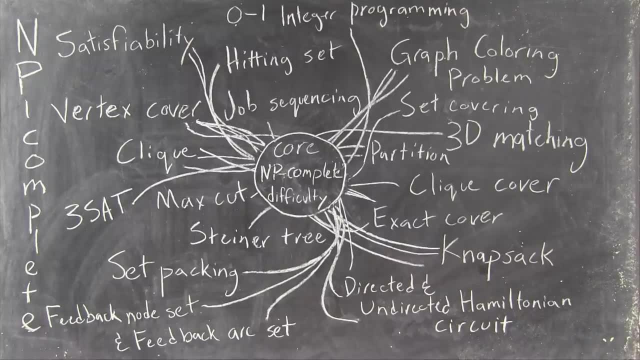 NP problems they were struggling with were essentially all the same problem, with some polynomial time complications thrown in here and there. These are called NP-complete problems and since that first batch in the seventies we've added Sudoku and protein folding and problems underlying puzzles and games like Battleship. 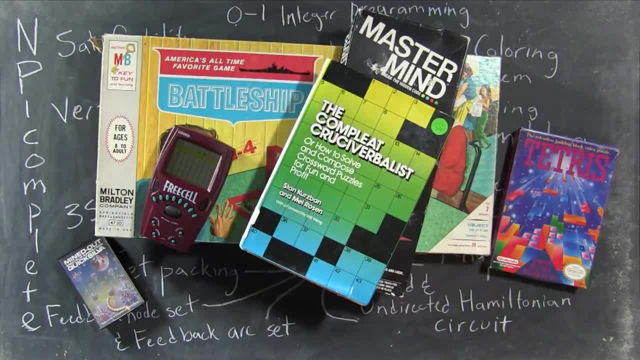 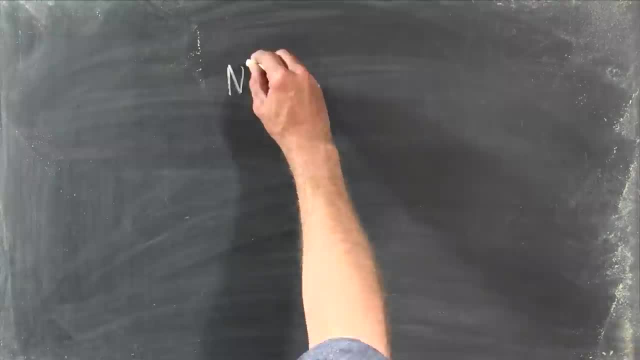 Free Cell, Mastermind, Tetris, Minesweeper and making up crossword puzzles. Even classic video games like Super Mario Bros and Metroid turn out to be connected to NP-complete level traversal problems. NP-complete is yet another math phrase, meaning that these problems include: 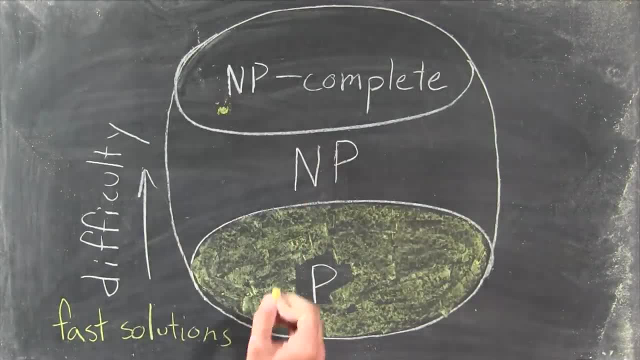 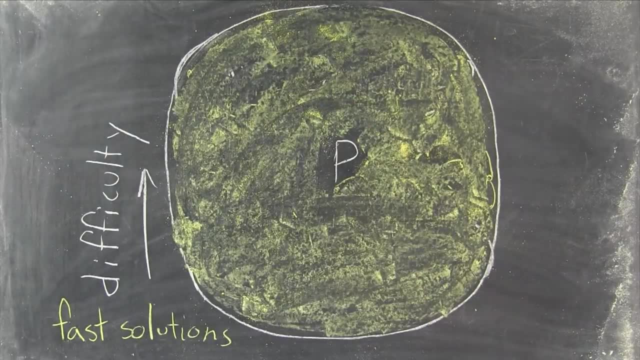 all the really hard parts of every NP problem. A fast program for solving any NP-complete problem would be used to solve every problem in NP. The whole class would instantly collapse. So yeah, amazingly, Sudoku is hard because it involves literally the same NP-complete. 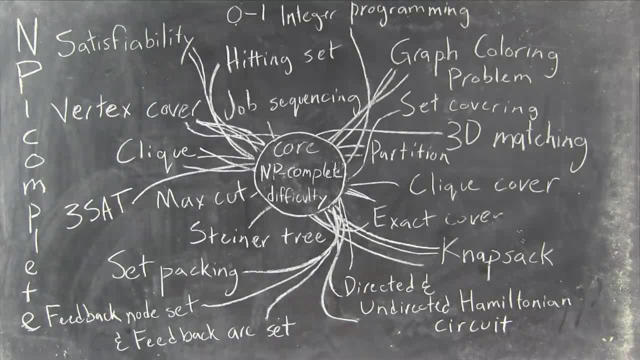 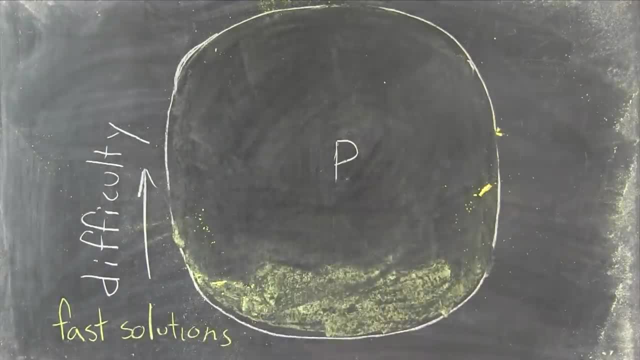 task that makes protein folding hard. If you come up with a profoundly faster way to play Sudoku, let somebody know. okay, Because fast protein folding would help us cure cancer. But the fact that a bunch of smart people have all been unsuccessful coming up with 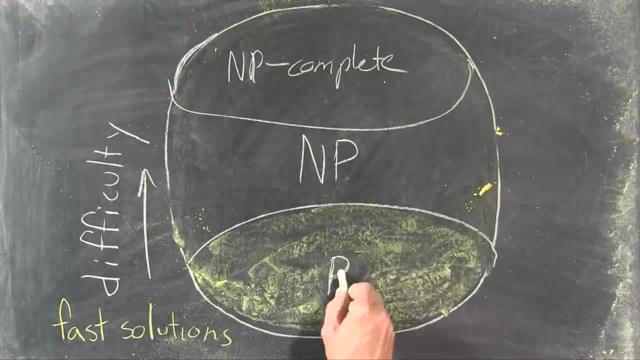 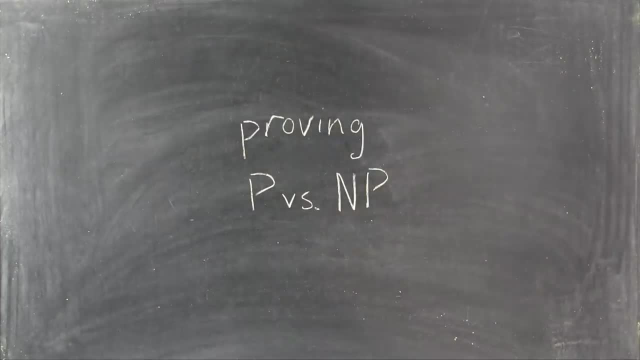 fast programs to solve what turned out to be essentially the same problem looks like a pretty good clue that the fast programs just aren't out there. So why has it been so hard to prove P versus NP? Well, fun fact, proving things is an NP problem. The P versus NP question itself is one of 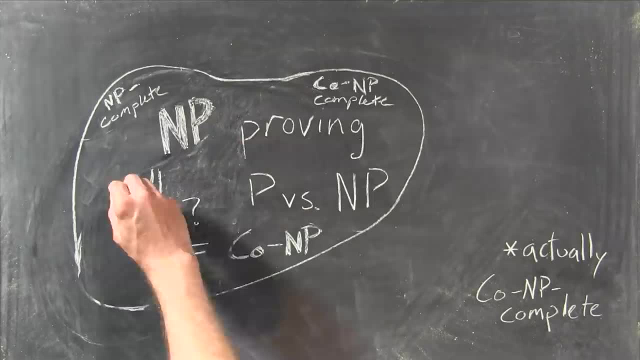 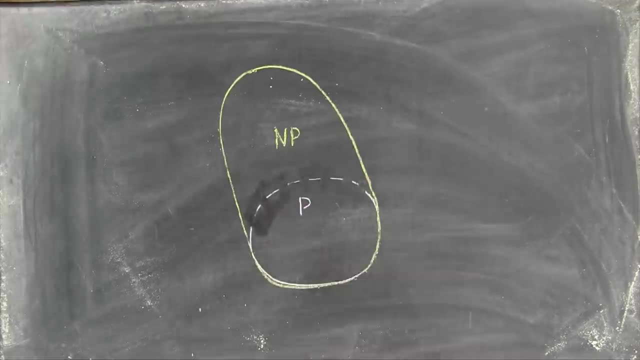 these problems. So yeah, this might be difficult Or not, We don't know. As the field of computational complexity has developed, we've discovered a lot of complexity. The P versus NP question turns out to be just the main attraction in a huge and complicated. 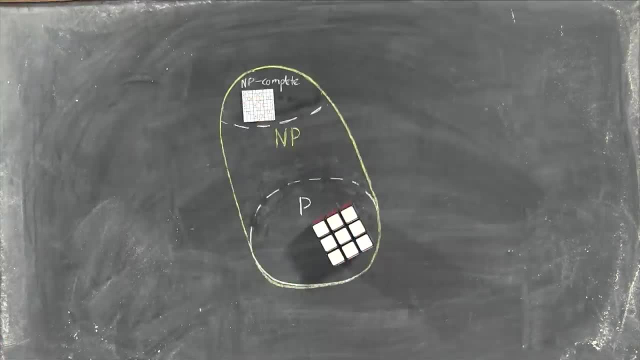 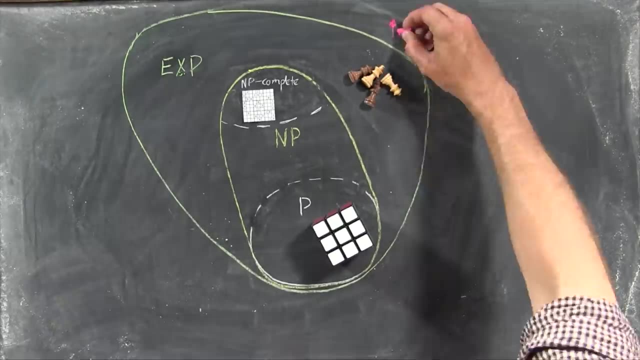 zoo of complexity classes. Beyond NP there are even harder classes of problems, like EXP, the class of problems including figuring out the best move in chess that takes exponential time to even check. This whole upper area of problems that are at least as hard as NP-complete is called NP-hard. There's also co-NP, the class of problems where, instead 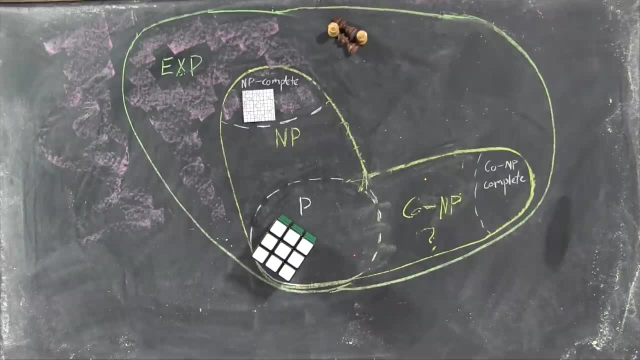 of being easy to check right answers, it's easy to exclude wrong answers, which may or may not be the same as NP. And then there's PSPACE, the class of problems that can be solved given unlimited time but using only a polynomial amount of space for memory. There, 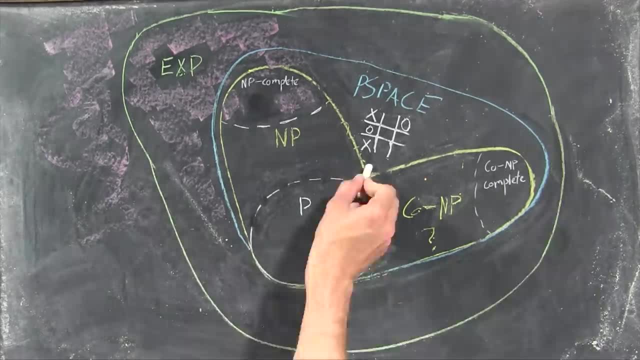 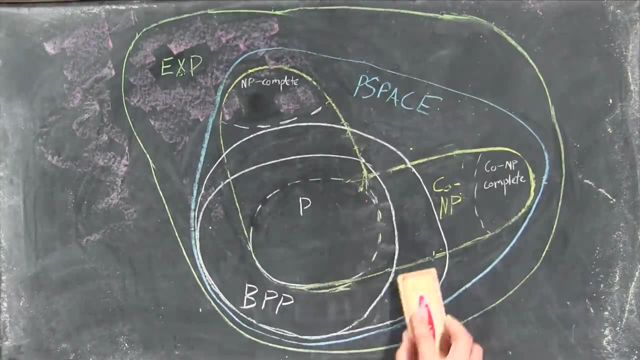 are also problems that can be solved probabilistically in polynomial time. That class is called BPP, and it may or may not actually be the same as P. And then there's a quantum computing analog of BPP called BQP- All over the place in here. 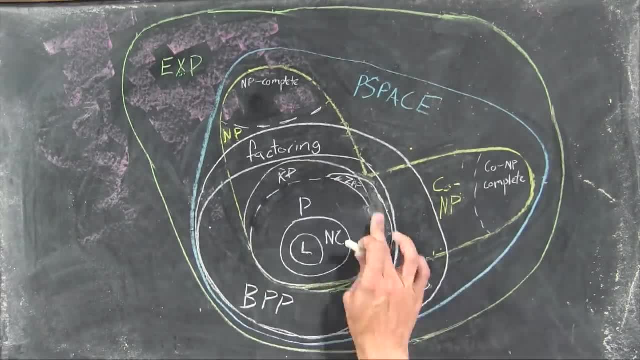 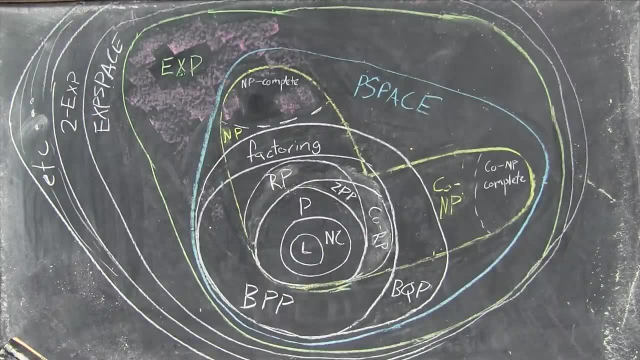 are complicated little classes that would take a lot of explaining, and actually some of these turn out to be infinite hierarchies of problems that are slightly more difficult from the ones beneath them. We know there's an exponential hierarchy and there's probably a polynomial hierarchy, And out beyond all of this are problems that are just not solvable. 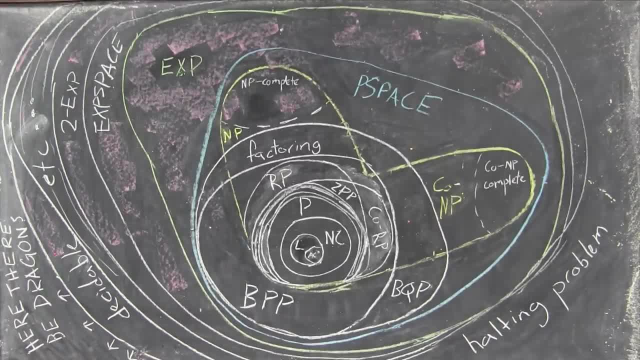 by any computer in any amount of time or space. To me, the amazing thing about this whole complexity zoo is that we're talking literally about what can be computed in a given amount of space and time. We're not just looking at the nature of computation here, we're looking at the nature of space. 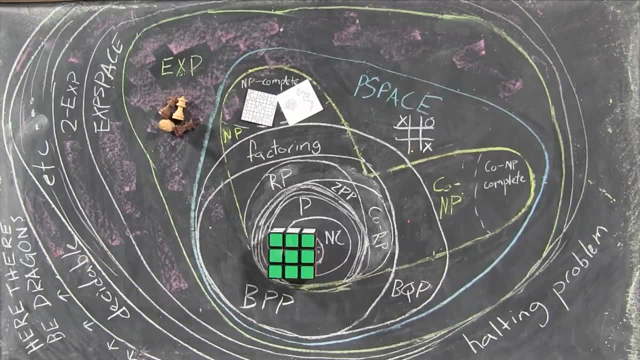 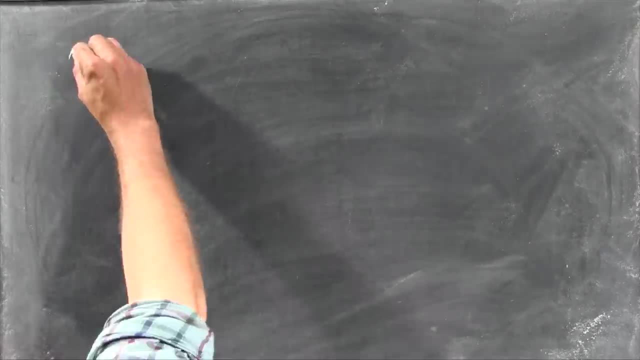 and time themselves. This mess of computational complexity classes, I think, ultimately has implications for physics and biology and for our basic understanding of everything. As an example of those implications, here's how Scott Aronson, a complexity researcher at MIT, explained his intuition about P versus NP. 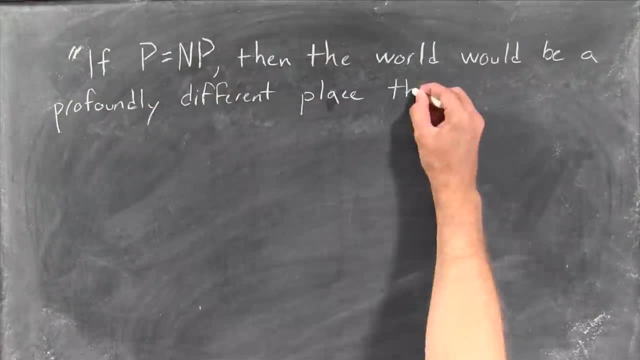 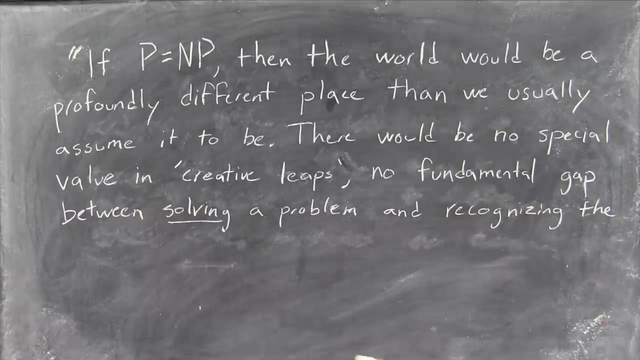 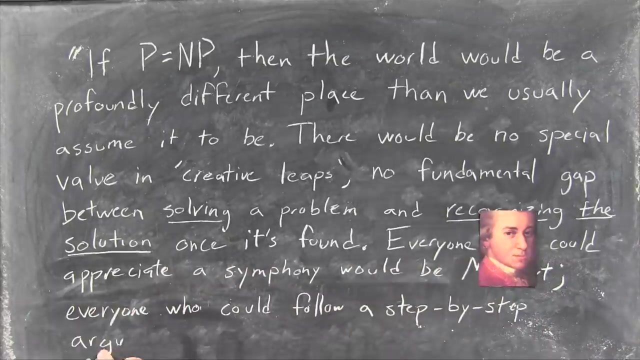 If P were equal to NP, then the world would be a profoundly different place than we usually assume it to be. There would be no special value in creative leaps, no fundamental gap between solving a problem and recognizing the solution once it's found. Everyone who could appreciate a symphony would be Mozart, Everyone who could follow a step-by-step. 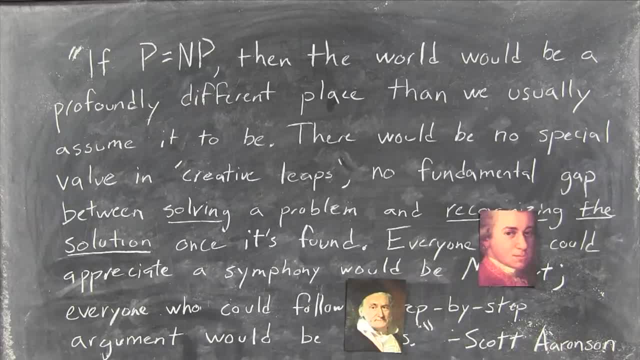 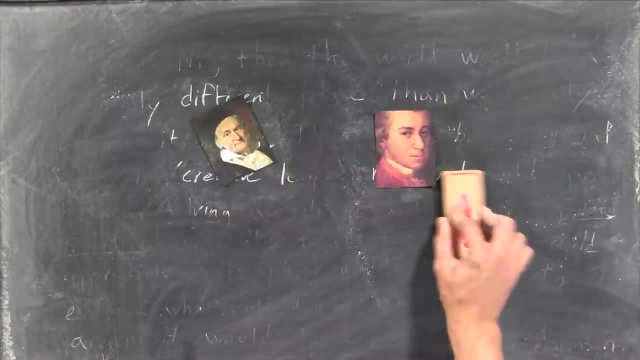 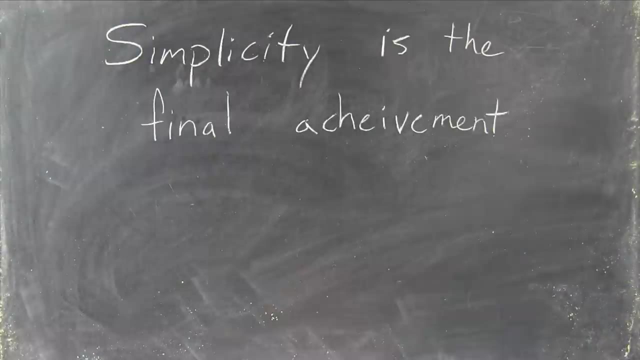 argument would be Gauss. The world around us, the nature of living things and ideas of art and genius is molded around the deep structure of computation In a very real way. something connected to P versus NP shows up in the struggles of scientists and artists. Chopin once said: simplicity is. 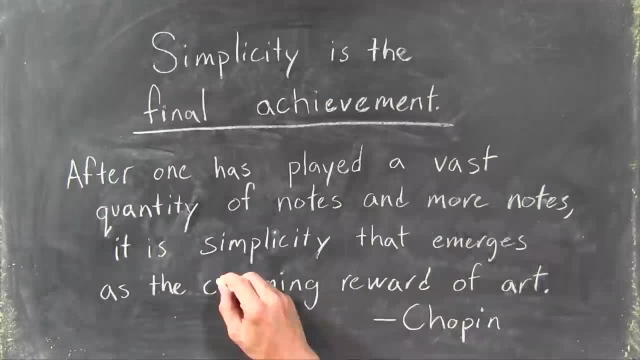 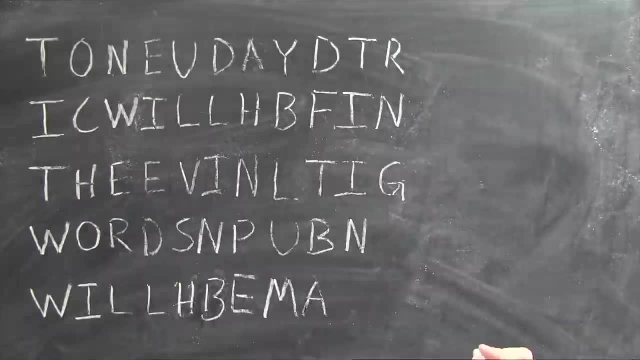 the final achievement. Despite a vast quantity of notes and more notes, it is simplicity that emerges as the crowning reward of art, And Jack Kerouac put it like this: One day I will find the right words, and they will be simple.